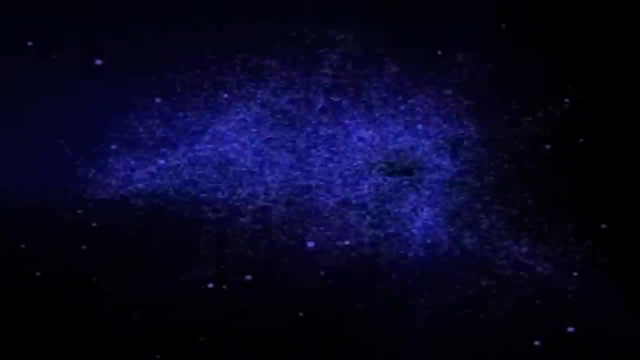 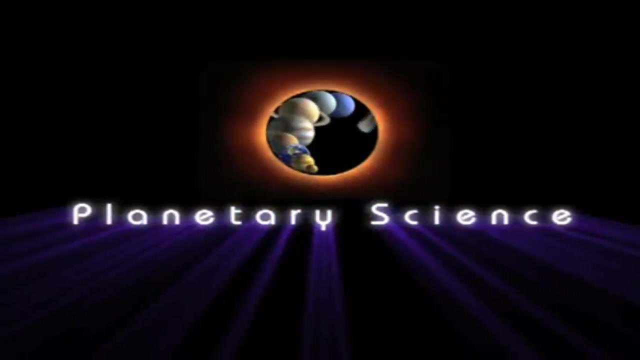 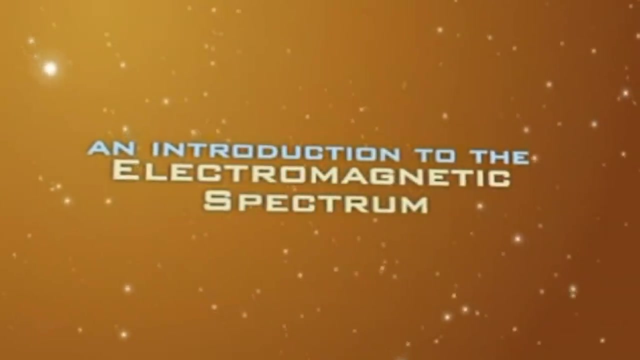 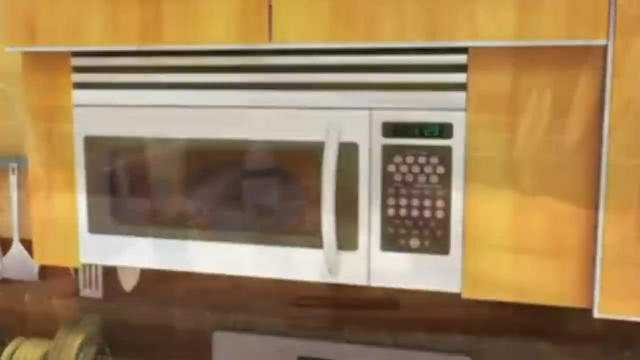 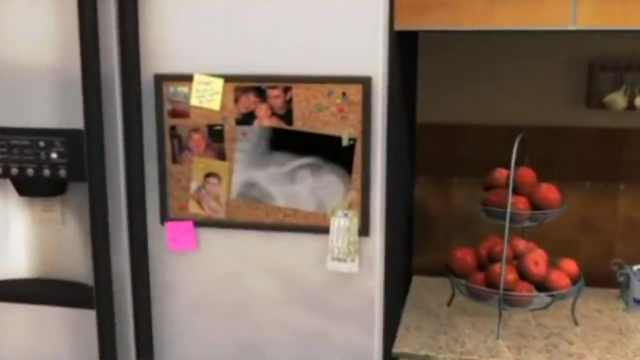 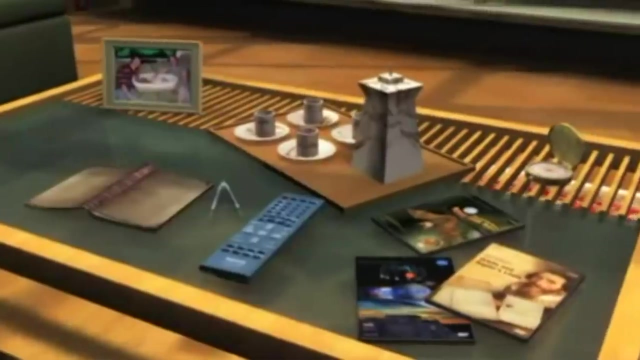 Something surrounds you, Bombards you, Some of which you can't see, touch or even feel Every day, Everywhere you go. It is odorless and tasteless, Yet you use it and depend on it every hour of every day. Without it, the world you know could not exist. 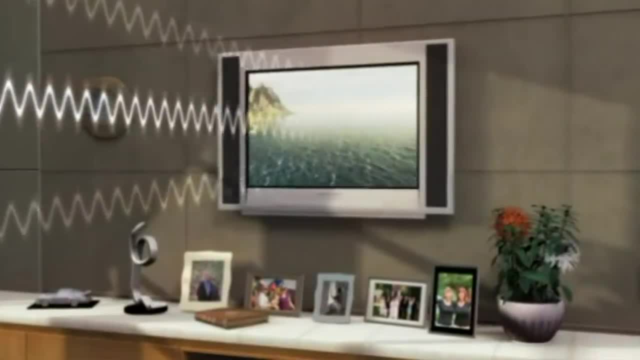 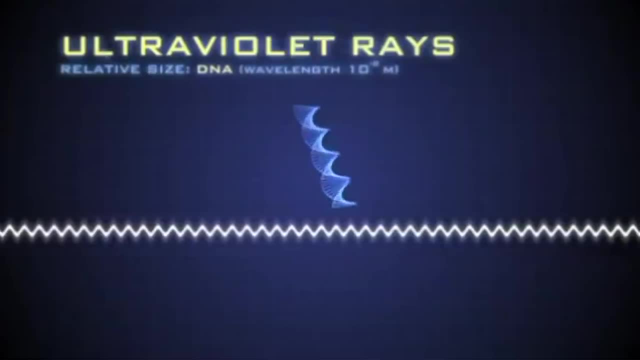 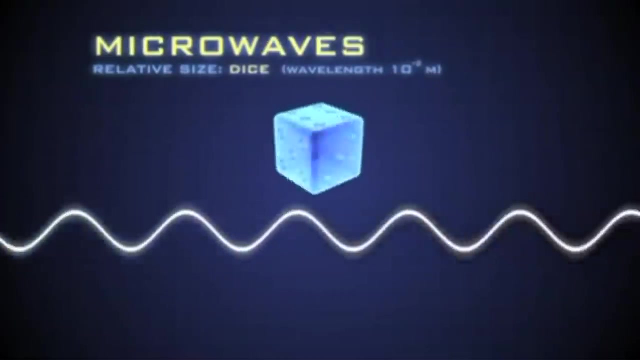 What is it? Electromagnetic radiation? These waves spread across a spectrum from very short gamma rays to X-rays, ultraviolet rays, visible light waves, Even longer infrared waves, Microwaves To radio waves which can measure longer than a mountain range. 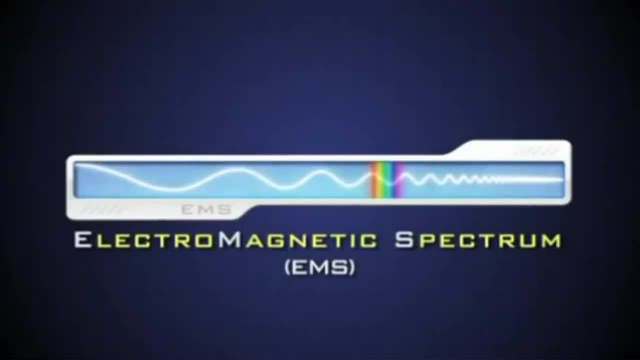 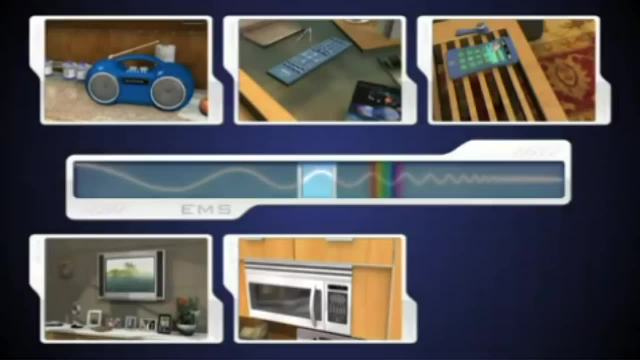 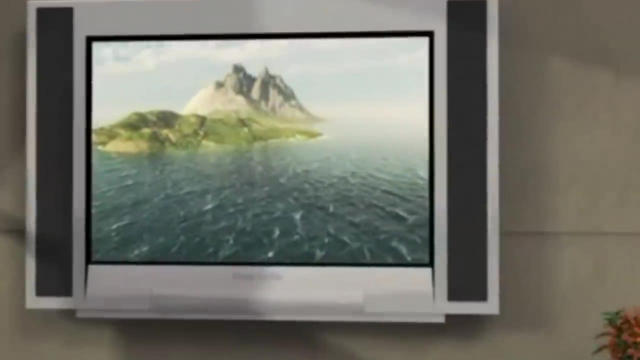 This spectrum is the foundation of the information age and of our modern world. Your radio remote control, text message, television, microwave oven, even a doctor's X-ray- all depend on waves within the electromagnetic spectrum. Electromagnetic waves, or EM waves, are similar to ocean waves in that both are 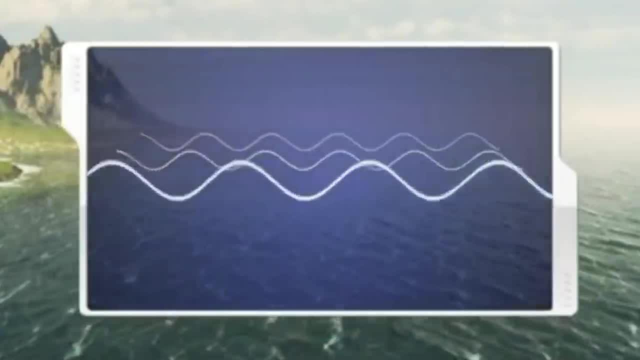 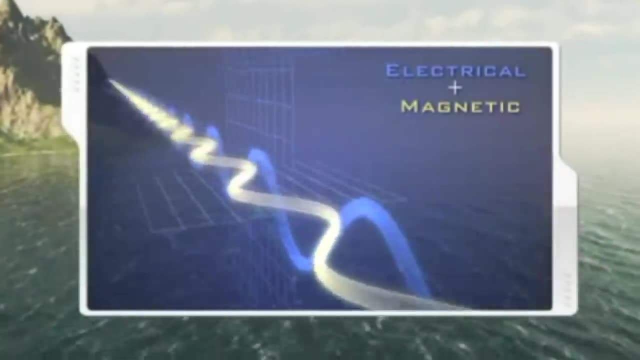 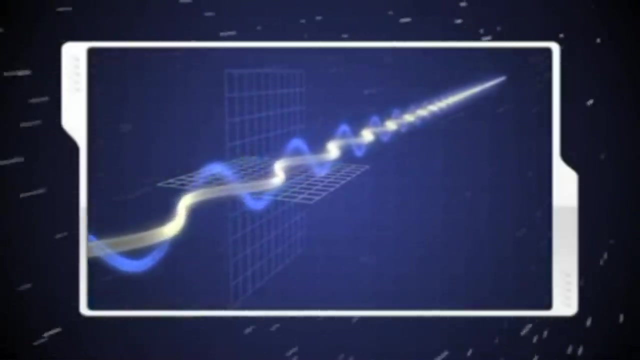 energy waves. They transmit energy. EM waves are produced by the vibration of charged particles and have electrical and magnetic properties. But unlike ocean waves that require water, EM waves travel through the vacuum of space at the constant speed of light. EM waves have crests and troughs like ocean waves. 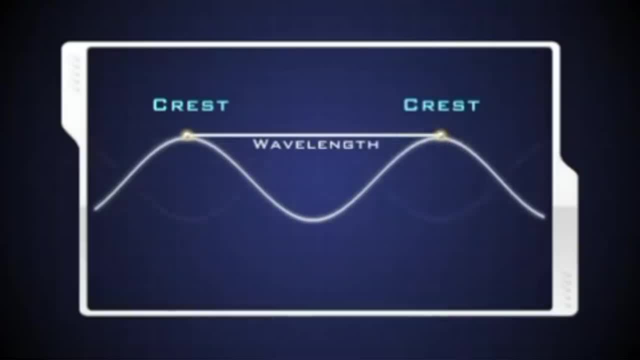 The distance between crests is the wavelength. While some EM wavelengths are very long and are measured in meters, The distance between crests is the wavelength. While some EM wavelengths are very long and are measured in meters, The distance between crests is the wavelength. 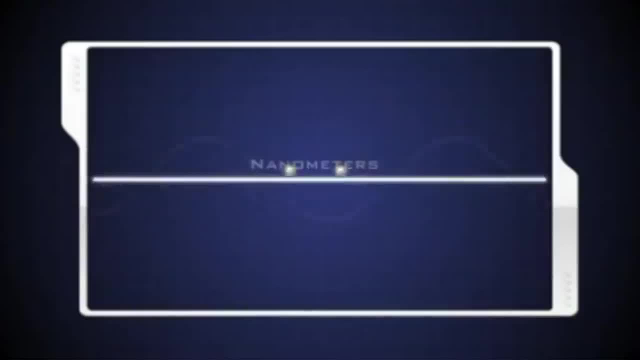 While some EM wavelengths are very long and are measured in meters, Many are tiny and are measured in billionths of a meter: nanometers. The number of these crests that pass a given point within one second is described as the frequency of the wave. 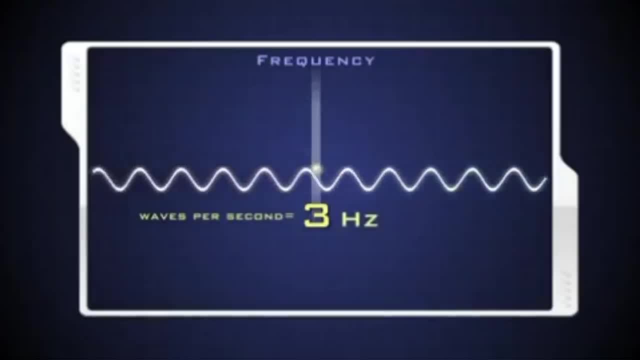 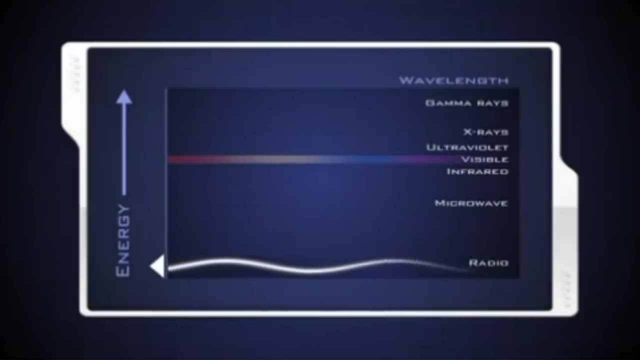 One wave or cycle per second is called a hertz Long. EM waves, such as radio waves, have the lowest frequency and carry less energy. Adding energy increases the frequency of the wave and makes the wavelength shorter. Gamma rays can also cause a couple of solar waves to show up at a time. 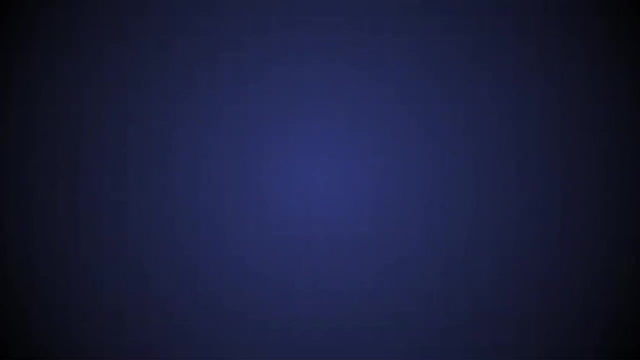 Gamma rays can also cause a couple of solar waves to show up at a time. As a result, gamma rays are the shortest highest energy waves in the spectrum. Gamma rays are the shortest highest energy waves in the spectrum. Gamma rays are the shortest highest energy waves in the spectrum. 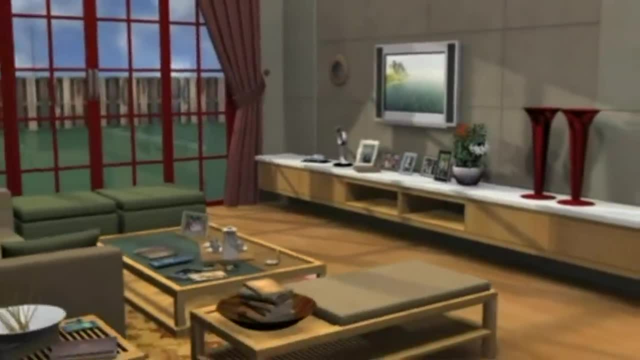 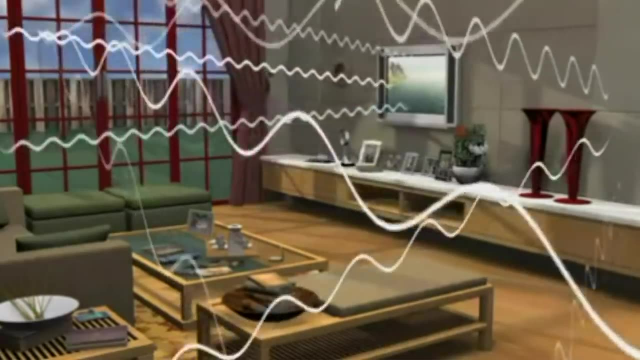 As you watch TV, not only are there light waves from the TV striking your eyes, but also radio waves transmitting from a nearby station and microwaves carrying telephone calls and text messages, and waves from your neighbor's Wi-Fi and GPS units in the cars. 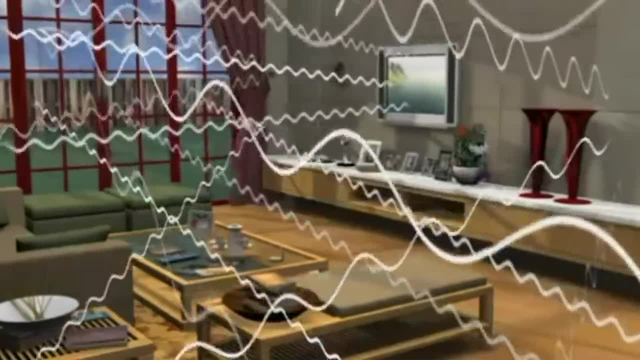 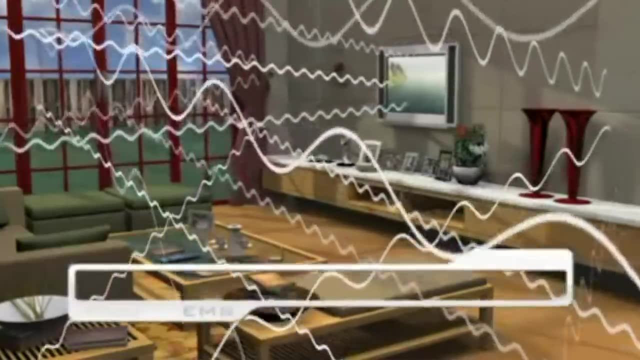 driving by. there is a chaos of waves from all across the spectrum passing through your room. right now, You can almost always run out of energy waves. as they pass by your doorsteps They can cause a fullupot of energy waves you how can you possibly watch your TV show? Similar to tuning a radio to a specific radio. 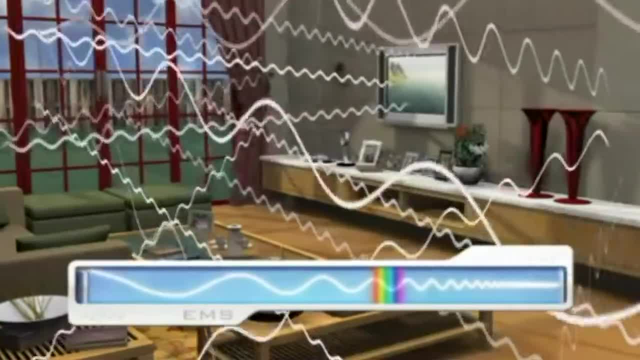 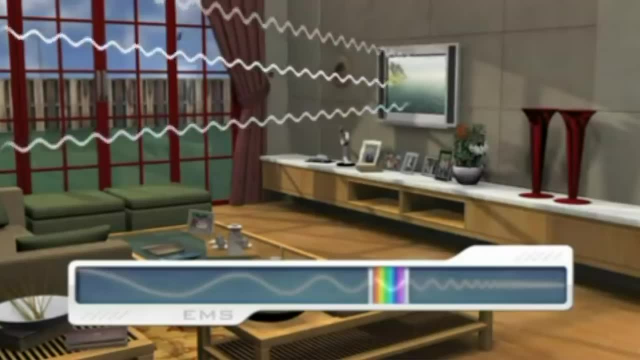 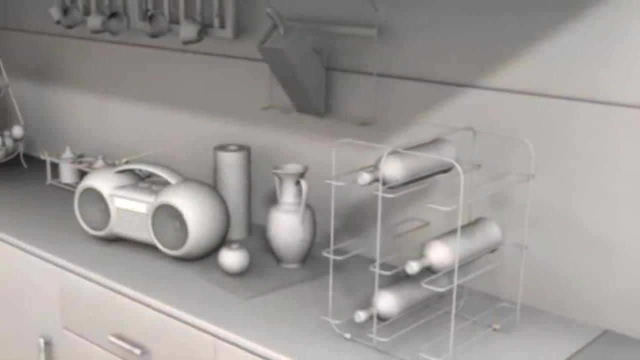 station. our eyes are tuned to a specific region of the EM spectrum and can detect energy with wavelengths from 400 to 700 nanometers, the visible light region of the spectrum. Objects appear to have color because EM waves interact with their molecules. Some wavelengths in the 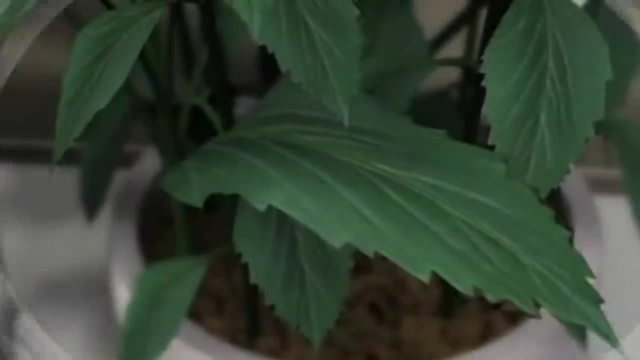 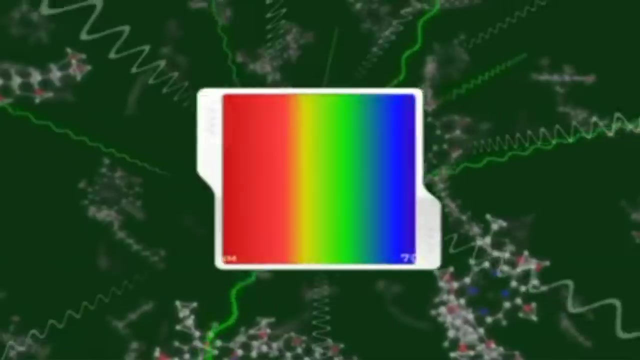 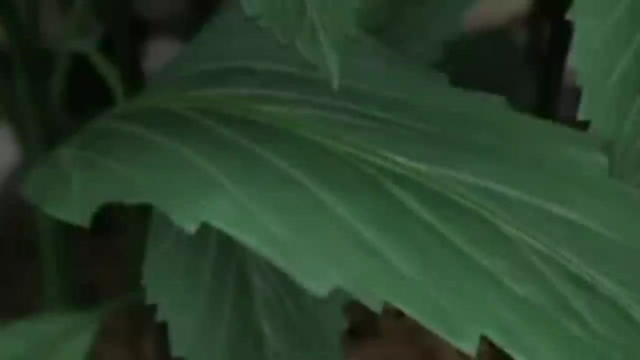 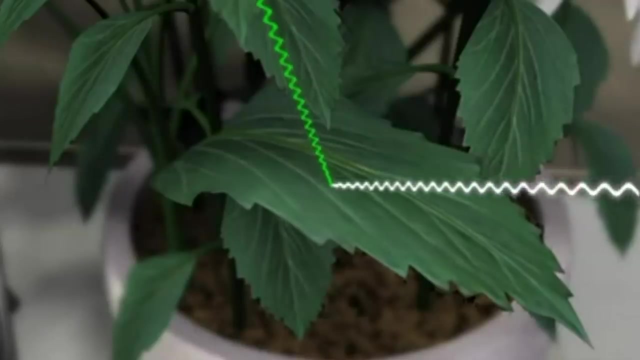 visible spectrum are reflected and other wavelengths are absorbed. This leaf looks green because EM waves interact with the chlorophyll molecules. Waves between 492 and 577 nanometers in length are reflected and our eye interprets this as the leaf being green. Our eyes see the leaf as green, but cannot tell us anything about how the leaf reflects ultraviolet. 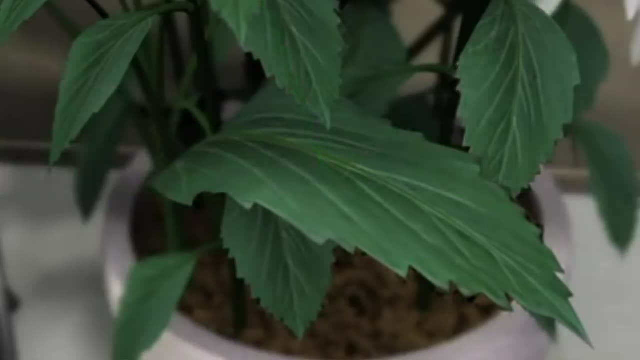 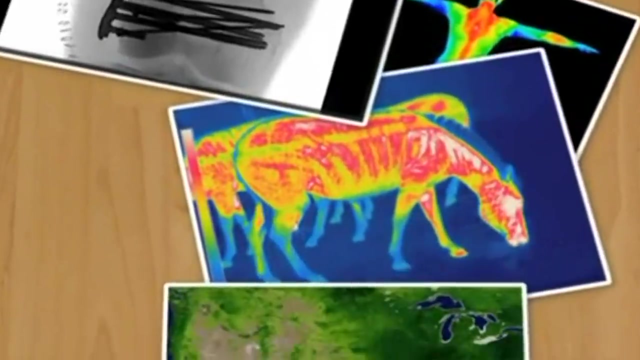 microwave or infrared waves. To learn more about EM waves, visit wwwemwavescom. To learn more about the world around us, scientists and engineers have devised ways to enable us to see beyond that sliver of the EM spectrum called visible light Data from multiple wavelengths. 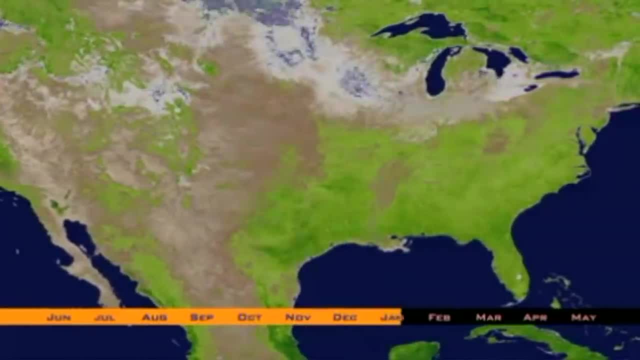 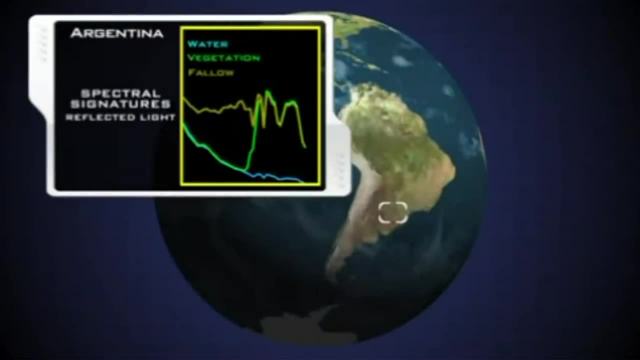 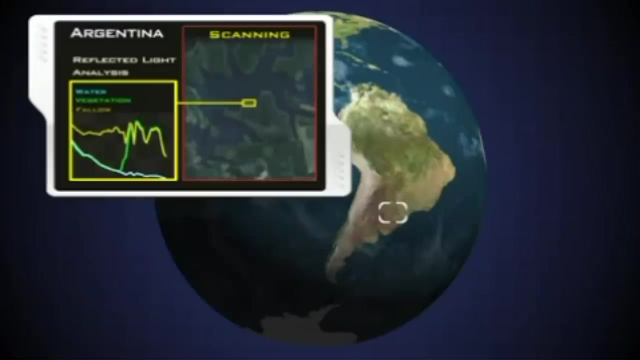 help scientists study all kinds of amazing phenomena on Earth, from seasonal change to specific habitats. Everything around us emits, reflects and absorbs EM radiation differently based on its composition. A graph showing these interactions across a region of the EM spectrum is called a spectral signature: Characteristic patterns like fingerprints within the spectra. 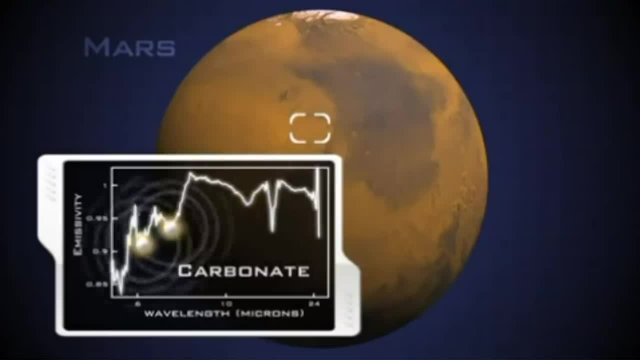 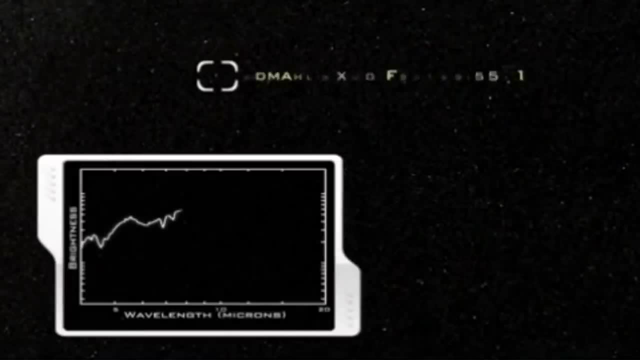 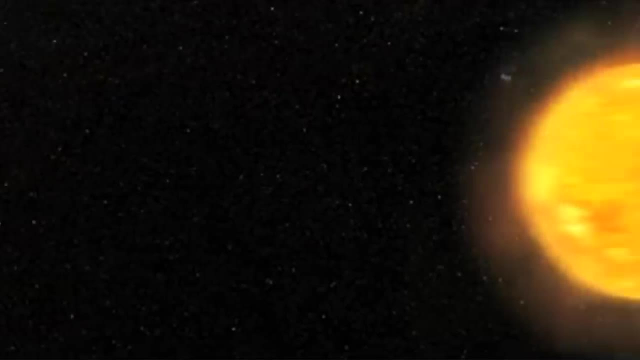 allow astronomers to identify an object's chemical composition and to determine such physical properties as temperature and density. NASA's Spitzer Space Telescope observed the presence of water and organic molecules in a galaxy 3.2 billion light years away, Viewing our Sun in multiple